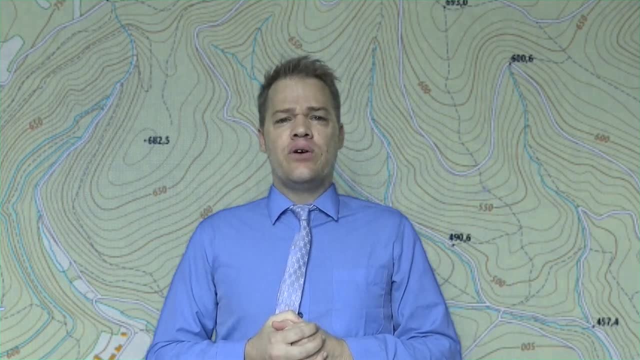 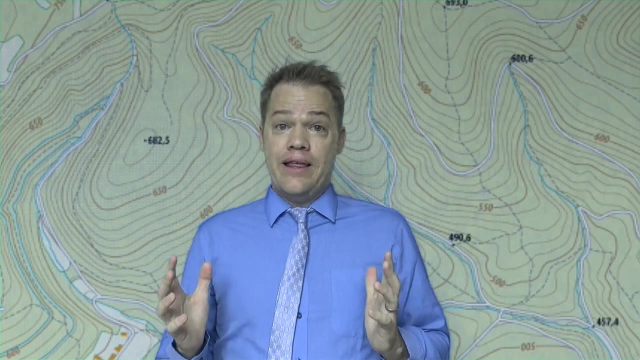 Hi and welcome once again to Channel Fish. In this video we are going to discuss the physical features that you typically see on topographic maps. So if you don't know anything about topographic maps yet, then I suggest that you go and watch the previous video I posted, where I 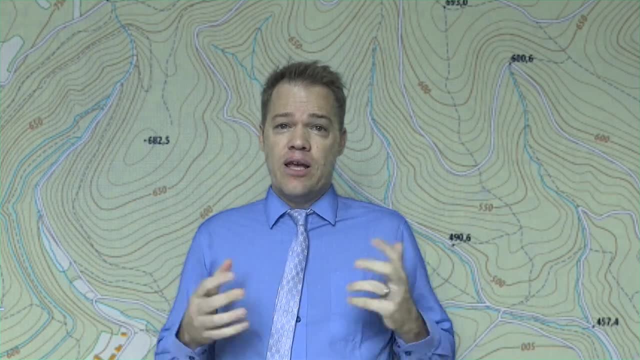 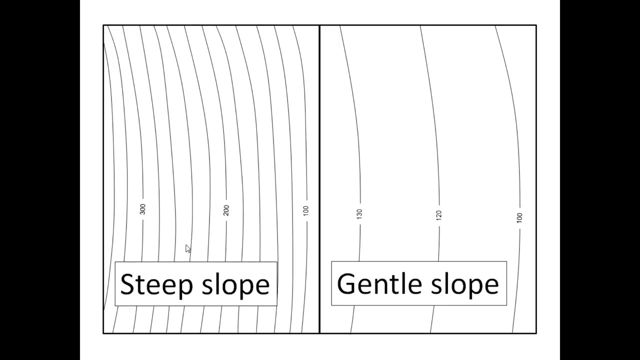 discuss the basics, But if you think you are familiar with the basics and if you think you have enough background knowledge, stay tuned. First thing we are going to look at are different types of slopes, and what is indicated on your left is a steep slope and on your right there's a gentle. 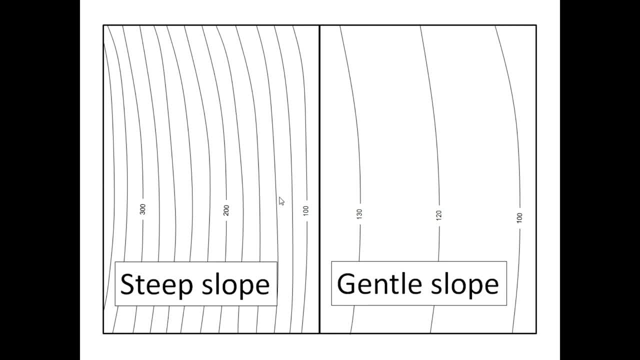 slope. So how do we know a slope is steep? It's when these contour lines are quite closely packed together. and it makes sense because if you look at the number 100 and this number 200, the contour interval here is 100 and this number 200 is 100.. So if you look at the number 100 and this number, 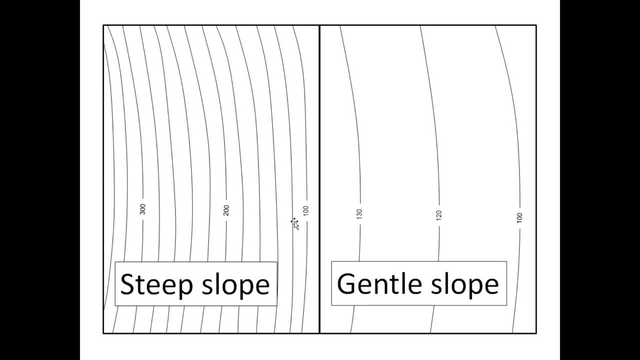 here, by the way, is 20.. So we go from 100 to 120 to 140, and it doesn't require us to go a long distance. So, in other words, we just travel a short distance in order to get to 120 meters, whereas 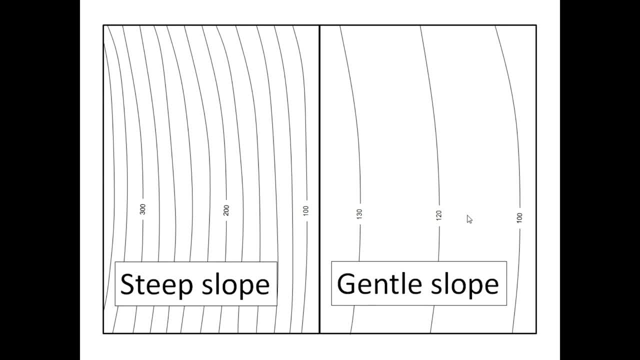 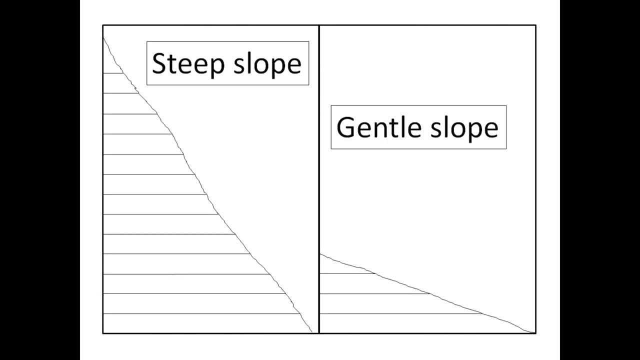 on this side, we see how we have to travel quite a long distance to get to the next level. So well, not the next level, but simply to 120 meters, and that is why it's a gentle slope. But I'm going to show you things from a different perspective. and so these contour lines, like we said, they connect places. 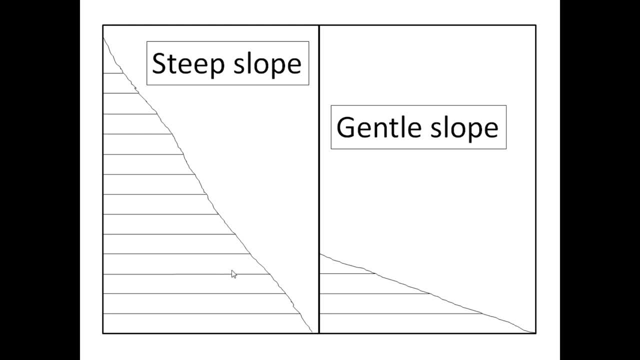 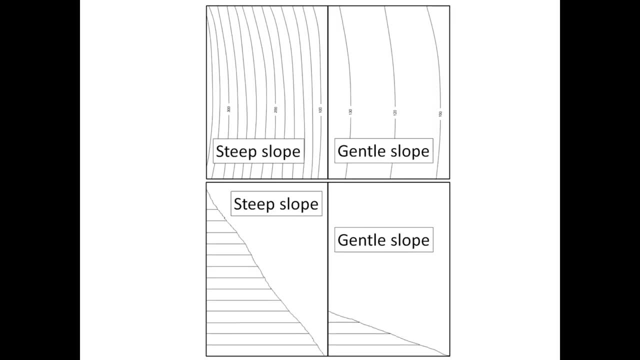 with exactly the same height, So they're always going to be straight when you look at it from the side or when you look at a cross section. And if you'd like to know what a cross section is and how to draw your own cross section, go look in the description where there's a link to one of my 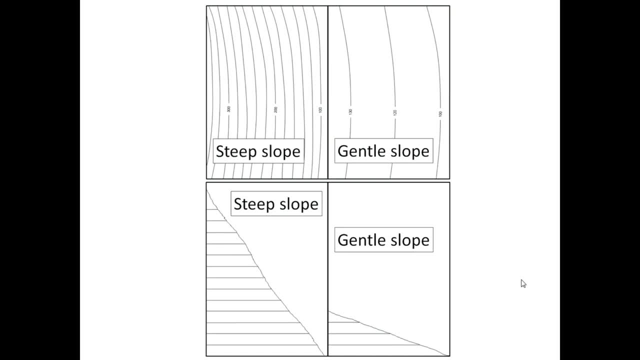 other videos where I explain step by step how to draw your own cross section. So this is a little bit of a detour, but I'm going to show you a little bit of a detour. So if you see, this is not an exact cross section of this contour map that you see over here, It's just to. 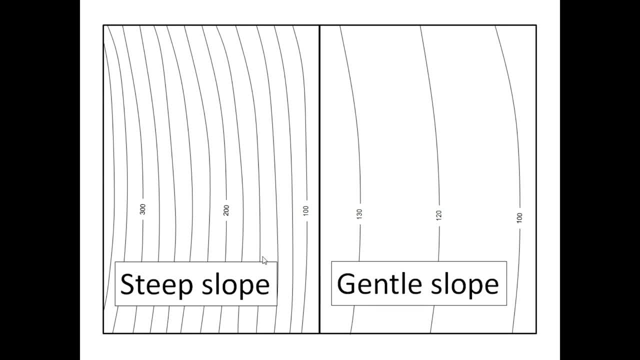 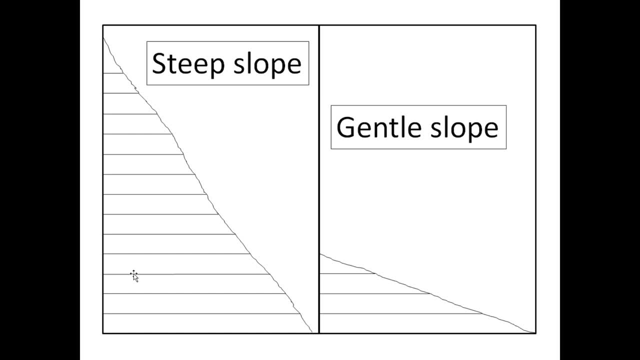 120 meters and that is why it's a gentle slope. but I'm gonna show you things from a different perspective. and so these contour lines, like we said, they connect places with exactly the same height, so they're always going to be straight when you look at it from the side or when you look at a cross-section. and if you'd 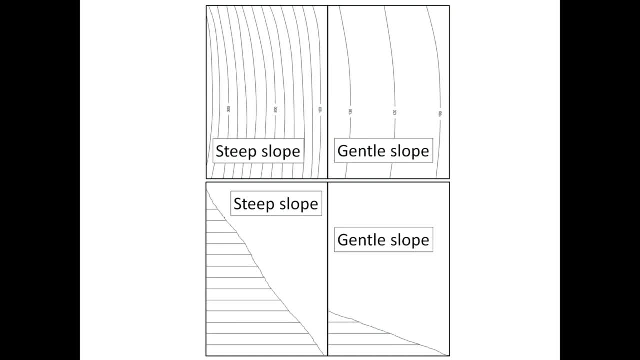 like to know what a cross-section is and how to draw your own cross-section? go look in the description, where there is a link to one of my other videos where I explain step by step how to draw your own cross-section. so this is not an exact cross-section of this contour map that you see over here. it's. 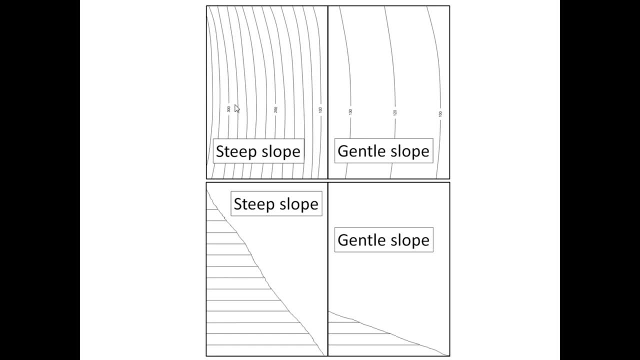 just to give you an idea. it's more or less, but not exactly the same, and so here we can see the lines quite closely packed together. that's why we have a steep slope, but there the lines are further spread apart, and that's why we have a gentle slope. 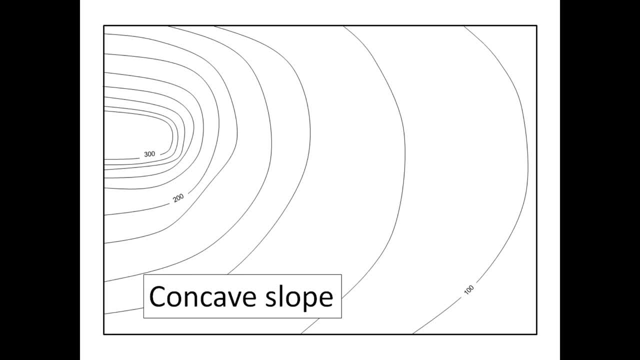 and so here we see a concave slope. the concave slope is a slope where you have contour lines far apart, at the bottom of the slope, or let's say at the foot of the mountain or the hill, and as we go higher they are more densely packed. 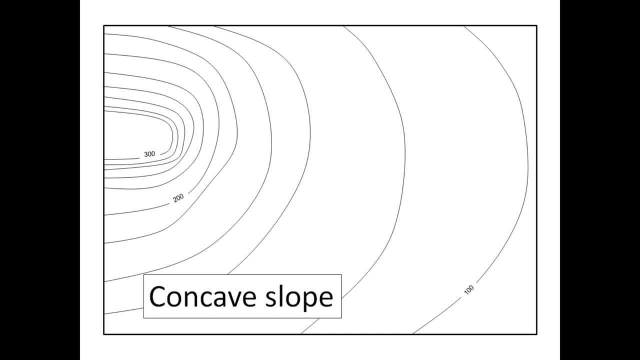 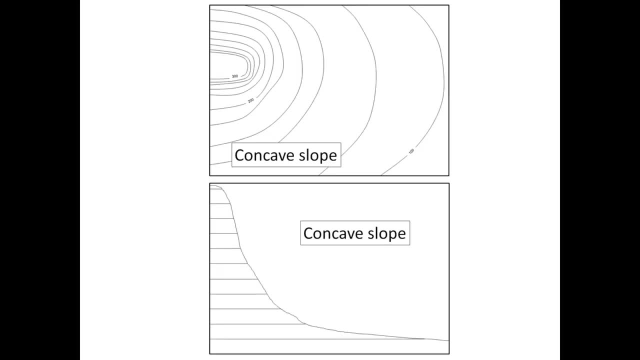 together, and so concave slope looks like this from the side. there you can see the concave slope from the side. and let's look at the two sides of the concave slope pictures put together. as we can see there they- they start out wide at the bottom. 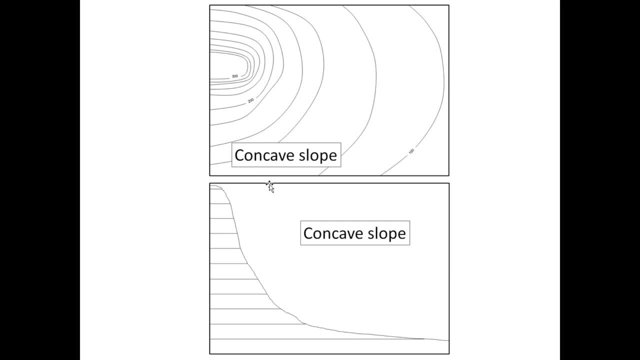 and then they, they're more densely packed as we go to the top, and i remember my teacher told me how to remember this- concave has an a and the a will help us there. these two lines are far apart at the bottom of the a, just like the contour lines, and as you go to the top uh, of the hill. 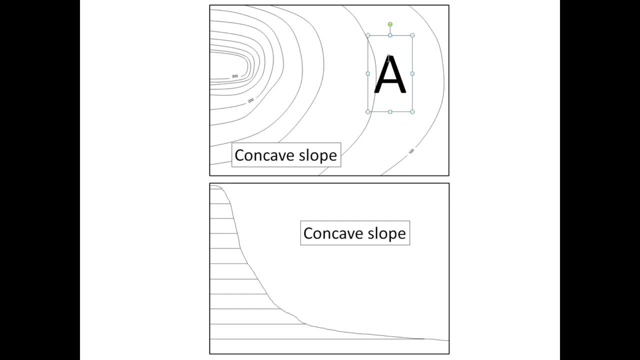 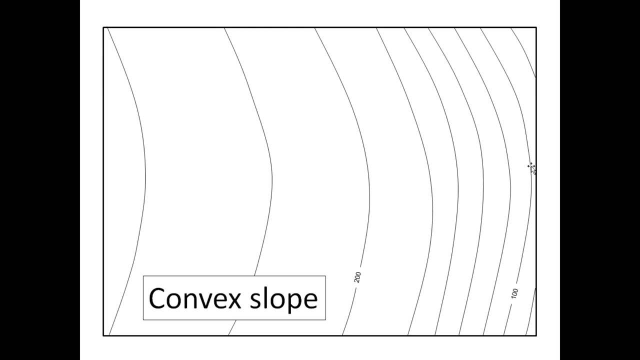 they are more closely packed. so these two lines come closer as we go to the top of the a and now we're going to move on to a convex slope. so a convex slope is a slope that has the contour lines closely packed at the bottom or at the foot of the hill or the mountain, and as we go to the top, 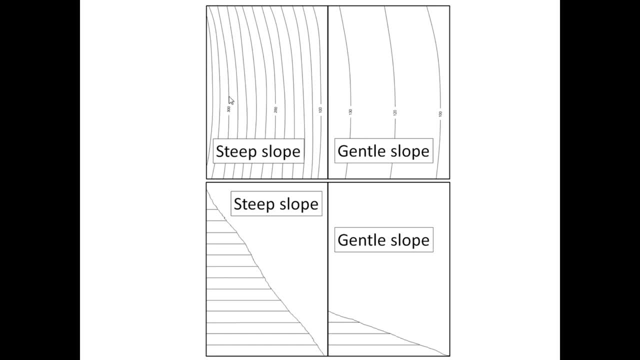 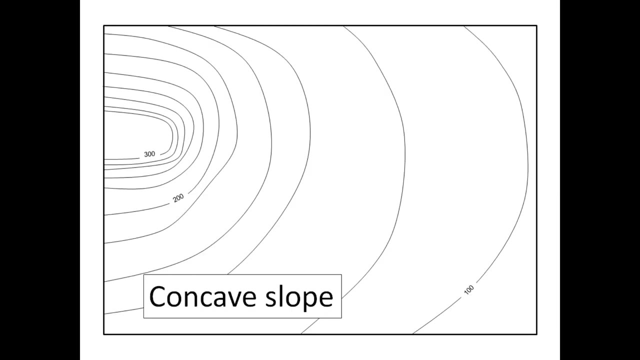 give you an idea. it's more or less, but not exactly the same. and so here we can see the lines quite closely packed together. That's why we have a steep slope, but there the lines are further spread apart, and that's why we have a gentle slope. And so here we see a concave slope. A concave slope is a slope where 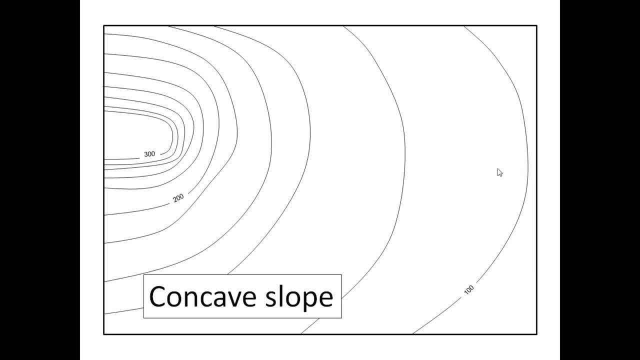 you have contour lines far apart, at the bottom of the slope or, let's say, at the foot of the mountain or the hill, and as we go higher they are more densely packed together, And so concave slope looks like this from the side. there you can see the concave slope from the side. Let's 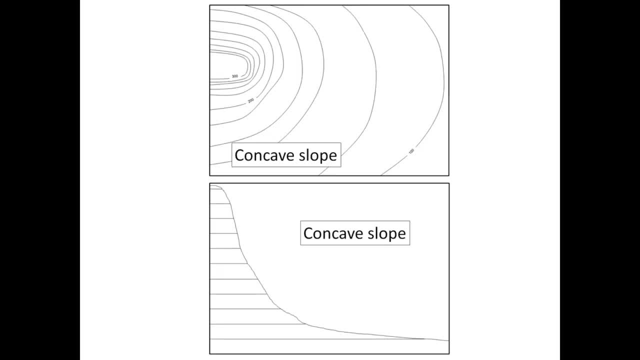 look at the two pictures put together, as we can see there they they start out wide at the bottom and then they are more densely packed as we go to the top. and I remember my teacher told me how to remember this concave has an A and the A. 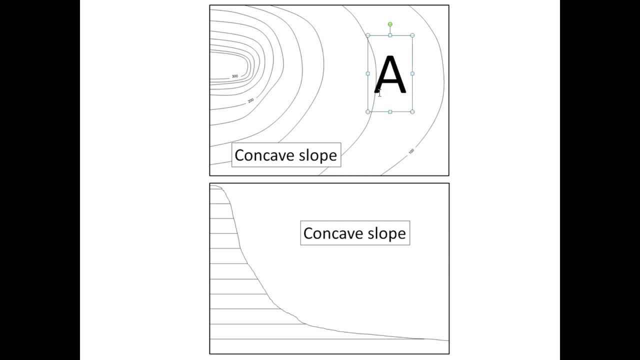 will help us there. these two lines are far apart at the bottom of the A, just like the contour lines, and as you go to the top of the hill they are more closely packed. so these two lines come closer as we go to the top of the A and 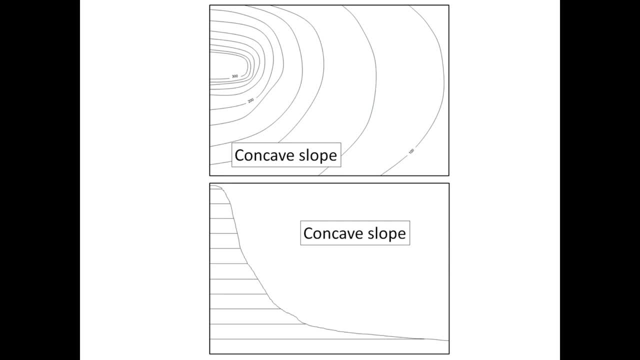 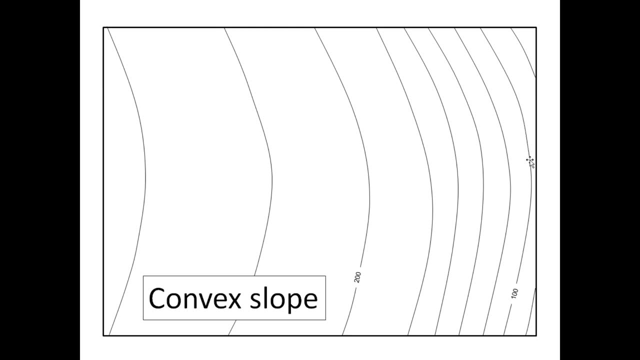 now we're going to move on to a convex slope. so a convex slope is a slope that has the contour lines closely packed at the bottom or at the foot of the hill or the mountain, and as we go to the top they are spread further apart, and so 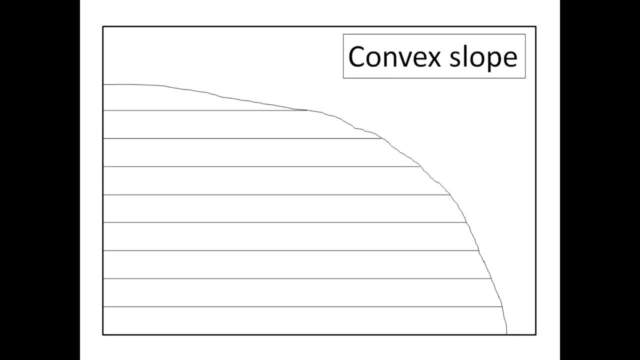 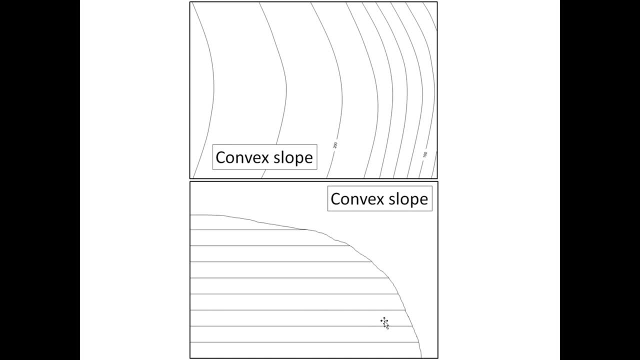 concave- sorry, a convex slope looks like this from the side of the A and then they are more densely packed. so these two lines come from the side and here's your two pictures put together. and how do we remember this? we use the A for concave. we're going to use a V for convex. so if 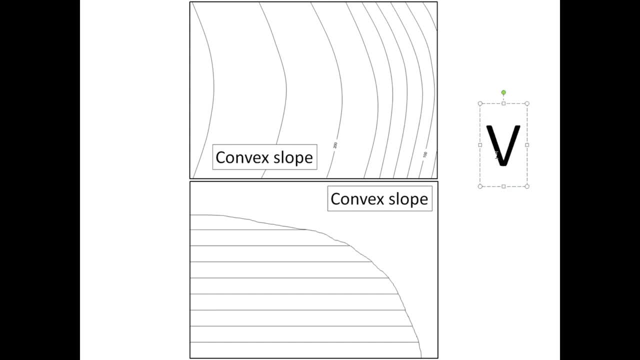 we look at this V, the two lines are close together. they even touch the at the bottom, but we're not going to focus on that. so the two lines are quite close together. at the bottom, the contour lines are closely packed at the bottom of the hill right and as we go to the top of the hill we're going to use a concave. 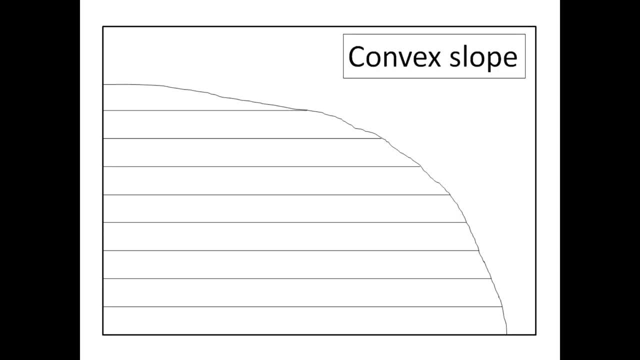 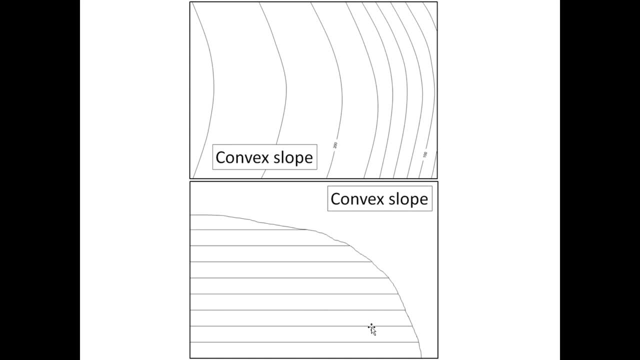 there are further apart and so concave- sorry, a convex slope looks like this from the side. and here's your two pictures put together. and how do we remember this? we use the a for concave. we're going to use a V for convex. so if we look at this V, 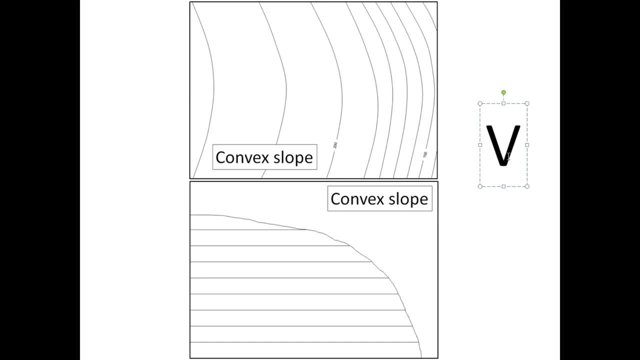 the two lines are close together. they even touch the at the bottom, but we're not going to focus on that. so the two lines are quite close together. at the bottom, the contour lines are closely packed at the bottom of the hill right, and as we go to the top of the hill they are spread out further. so it's the same. 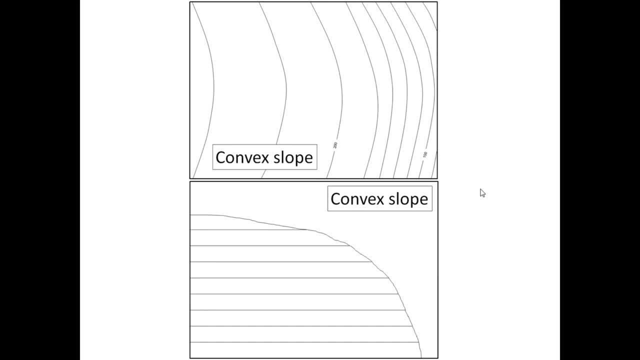 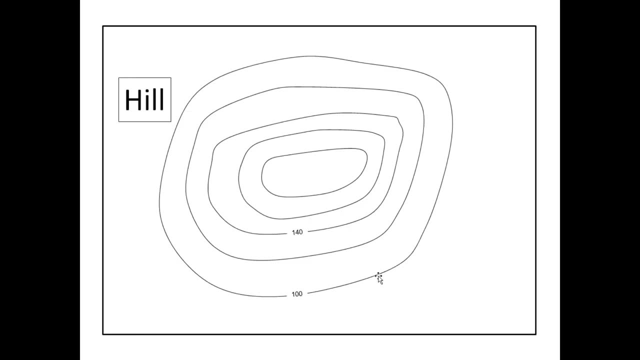 with the V, and that's how you remember the difference between convex and concave. now we're going to move on to a hill. so a hill is a very simple feature on a contour map or a topographic map. so it looks like this from the top: the circular. 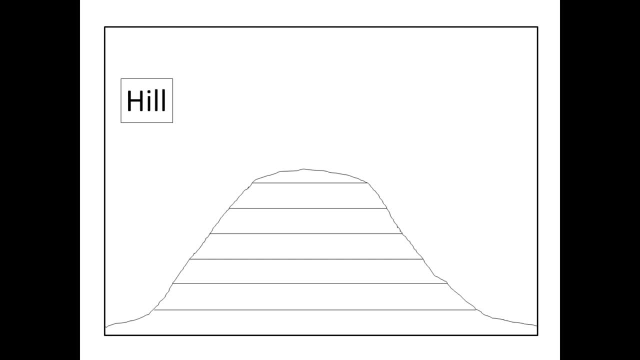 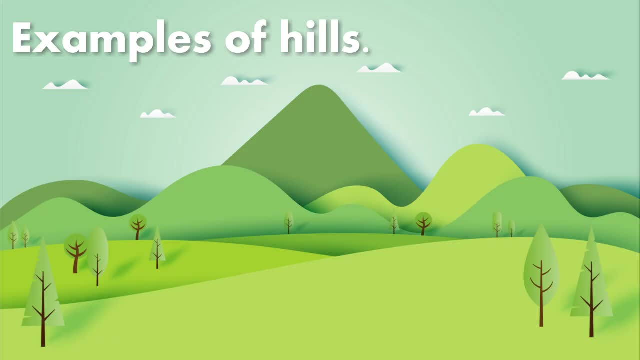 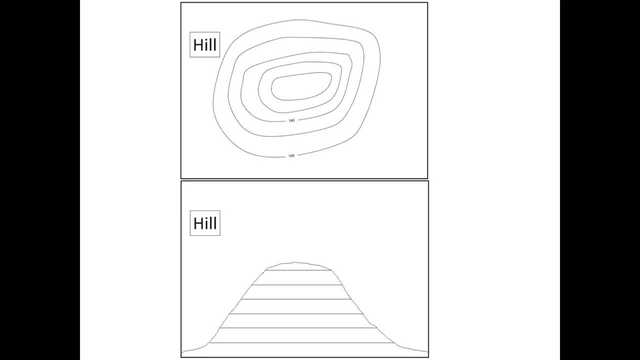 lines and then, if you look at it from the side, this is what it looks like. the cross-section effect looks like this. so I think by now, all of you should should have a feeling, or at least an idea, of how to interpret contour maps. when you look at it, what we have here is a valley, and this is an example of a valley. 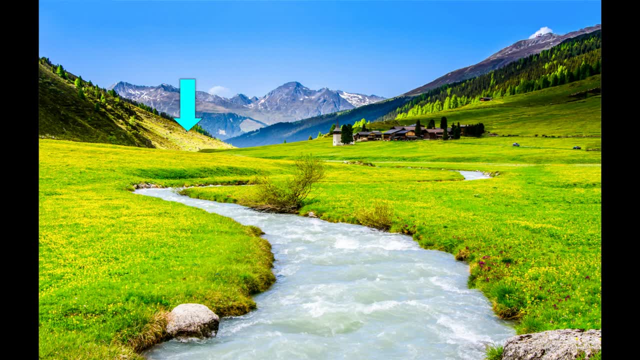 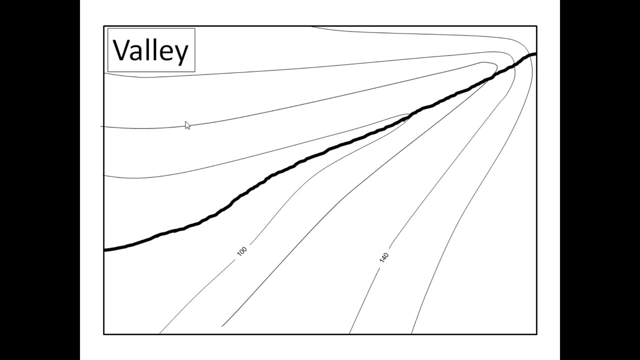 and actually, in transfer, I actually identified the value value of this and the vector value for this, so it provides us with real formula in terms of the depth and extent of these mountain points, as well as the depth of väldigt small mountain, and then also, what I would like you to pay attention, 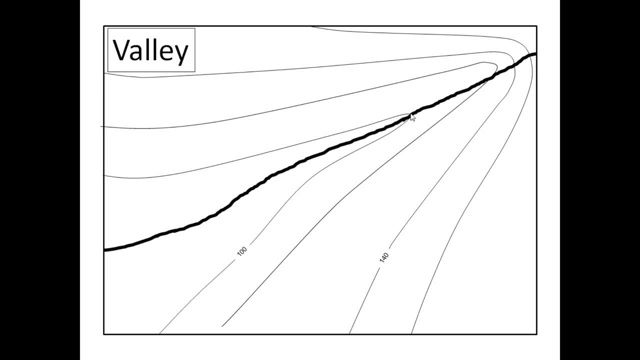 to are these bottom sections of the mountains, and these are called Spurs, and if the source of the river is up here, then the river will flow down in this direction. so here we have a hundred meters, 120, 140, so you can imagine how this land is shaped. now, please take note that when you look at these contour 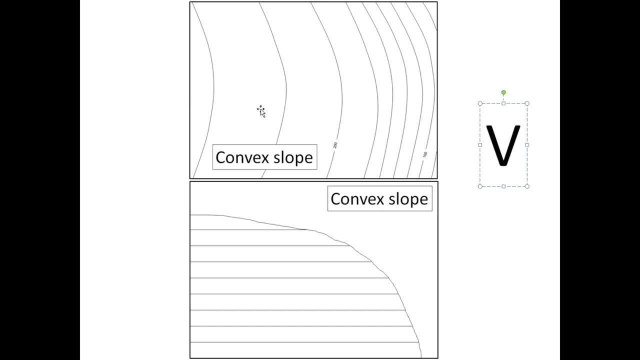 slope. so we're going to use a concave slope. so if we go to the top of the hill, they are spread out further. so it's the same with the V and that's how you remember the difference between convex and concave. now we're going to move on. 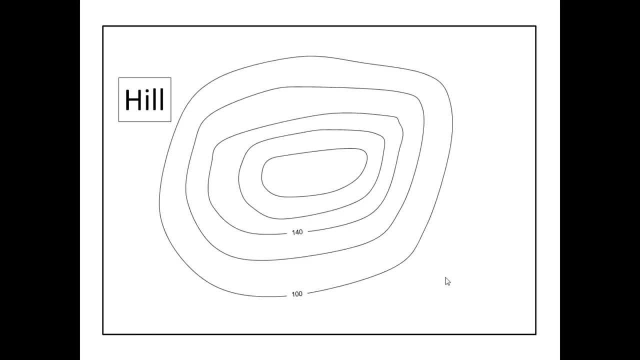 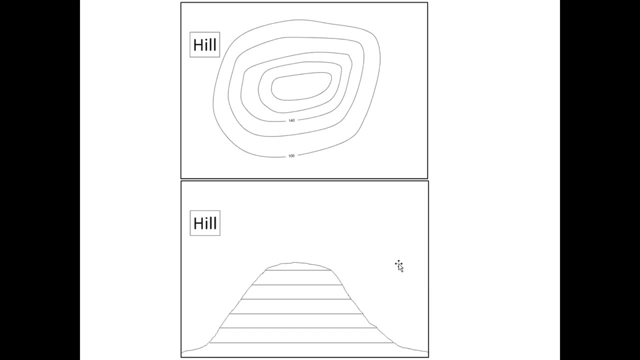 to a hill. so a hill is a very simple feature on a contour map or a topographic map. so it looks like this from the top, the circular lines, and then, if you look at it from the side, this is what it looks like. the cross-section effect looks like this. so I think by now all of you should 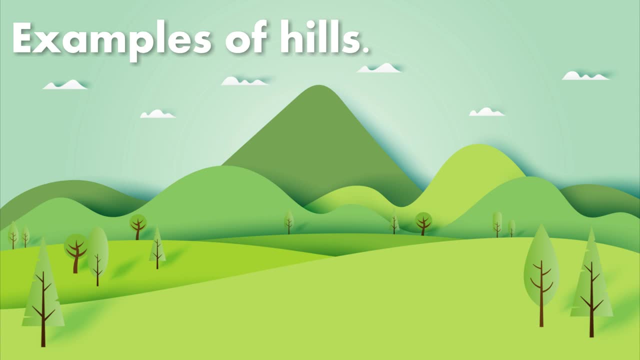 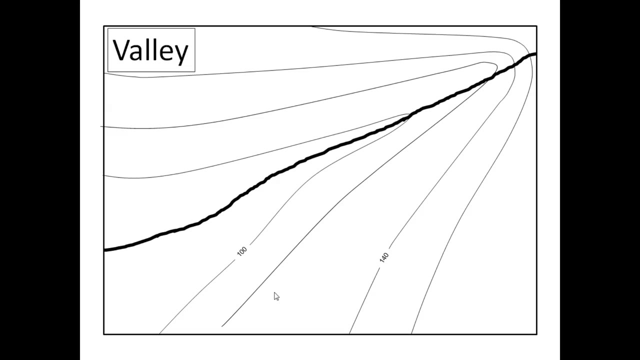 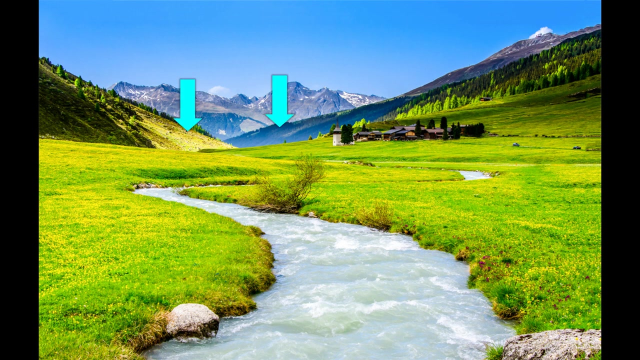 should have a feeling, or at least an idea, of how to interpret contour maps. when you look at it, what we have here is a valley, and this is an example of a valley. and then also, what I would like you to pay attention to are these bottom sections of the mountains, and these are called spurs. 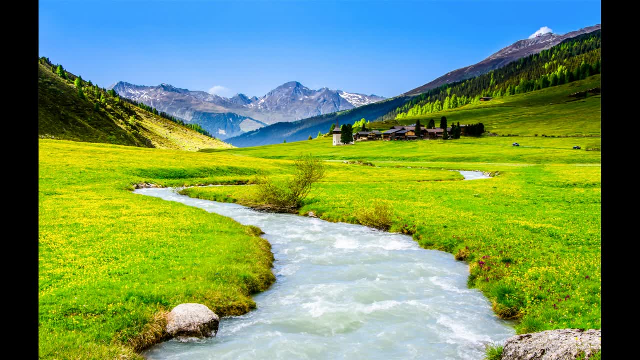 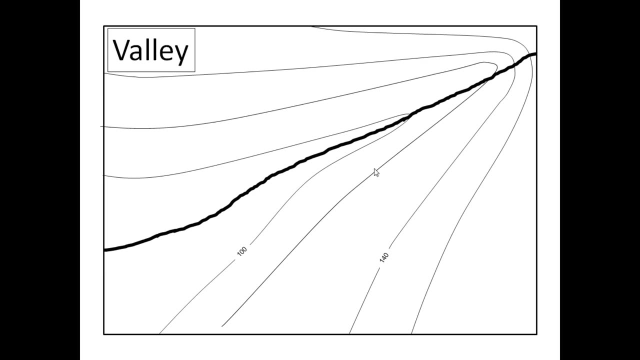 and we are going to discuss this topic later in the video. So what we have are these contour lines, and you can see they are forming a V right Now. the point of the V points to the source of the river. So if the source of the river is up here, 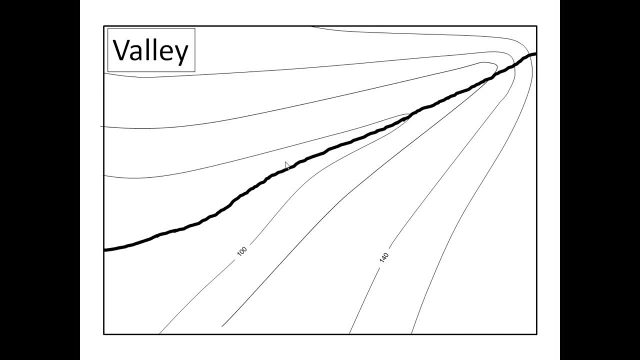 then the river will flow down in this direction. So here we have 100 meters, 120,, 140.. So you can imagine how this land is shaped. Now, please take note that when you look at these contour lines, you'll notice. 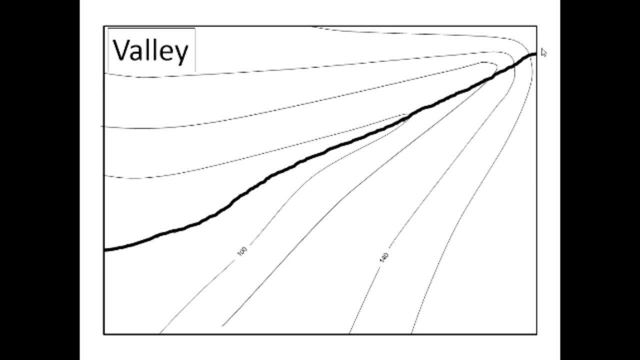 that they are reasonably close together, which means there is a steepish slope, and it tells us that it is the upper end of the valley. It's also called a young valley sometimes, But when we go down the river to the lower parts of the valley, 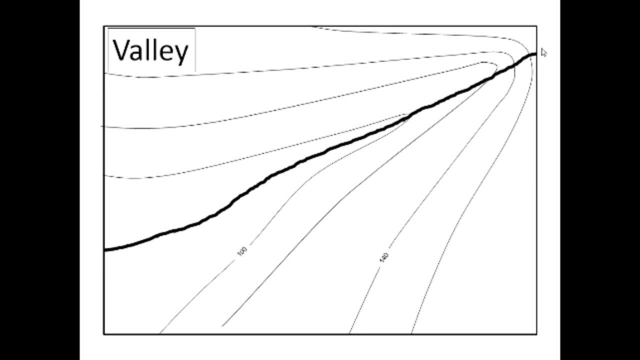 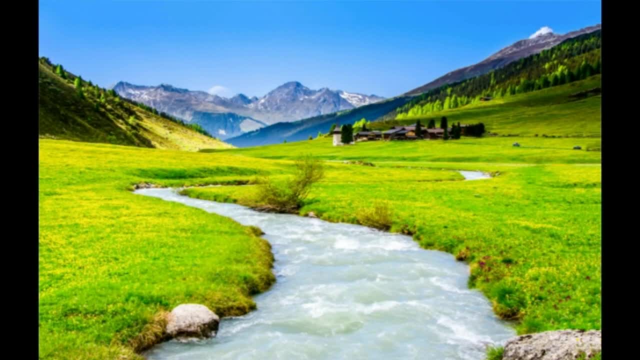 that's where we have a reasonably even surface. So, if we go back to the picture we saw earlier, this is a typical example, as I said, of a valley, And what you see on your screen is a contour map of a similar type of valley. 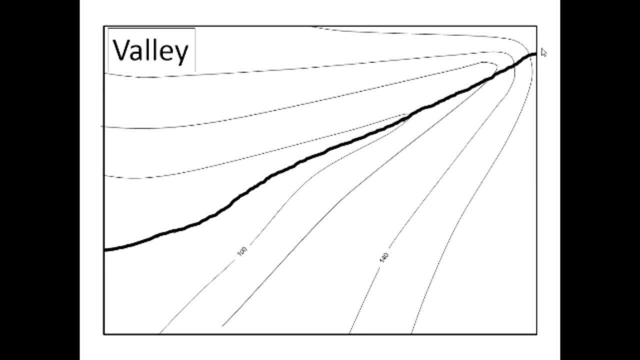 lines, you'll notice that they are reasonably close together, which means there is a steepish slope, and it tells us that it is the upper end of the valley. it's also called a young valley sometimes, but when we go down the river to the lower parts of the valley, that's where we have a reasonably even surface. 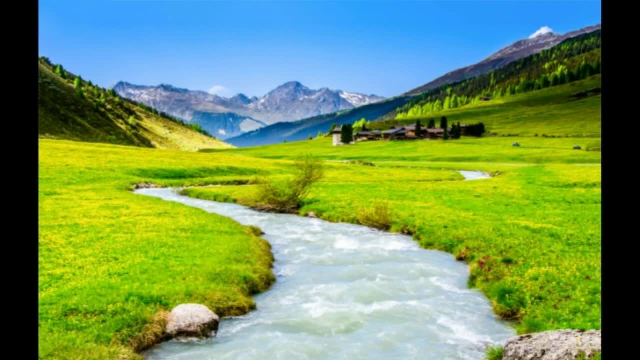 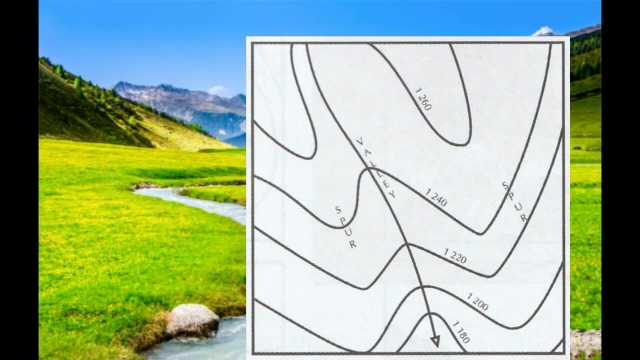 so, if we go back to the picture we saw earlier, this is a typical example, as I said, of a valley, and what you see on your screen is a contour map of a similar type of Valley. it's not the valley in the picture, it's just a very similar Valley in the sense that the slope is very 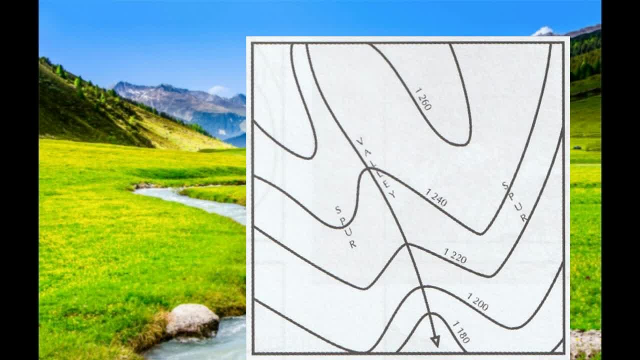 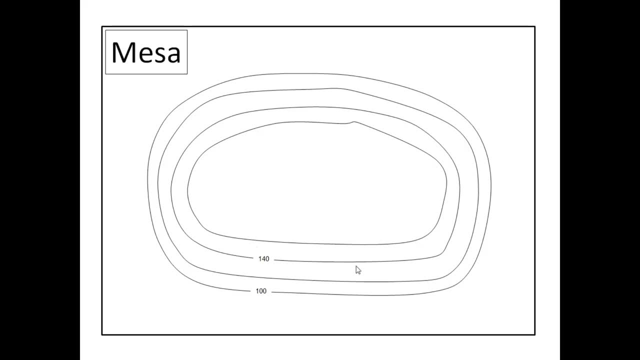 gentle, and the contour lines are more dispersed, so it might be slightly more challenging to identify a Valley where the lines are so dispersed. next we have a Mesa. now a Mesa is almost like a hill, but the top is flat, and there we see what the Mesa looks like at�34røёл34, but you will see how flat now the top is flat as Schwalbe, and hier we see what the這裡. 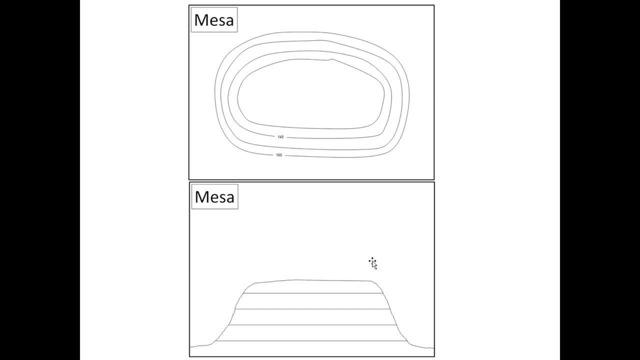 looks like from the side the. the cross-section perspective looks like this, and there you can see the top is quite flat, and what you should remember- something I haven't mentioned yet- is that if this is there, we see it 140. so this is 160. so if this line is 160 meters above sea level, then everything. 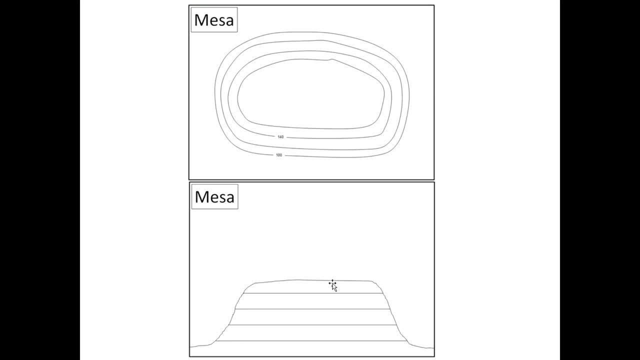 above this is below 180. and how do we know that? we know it because the contour interval is 20 meters, but we don't have another contour line above this one. so if this line is 160, then everything above this is higher than 160, but it's. 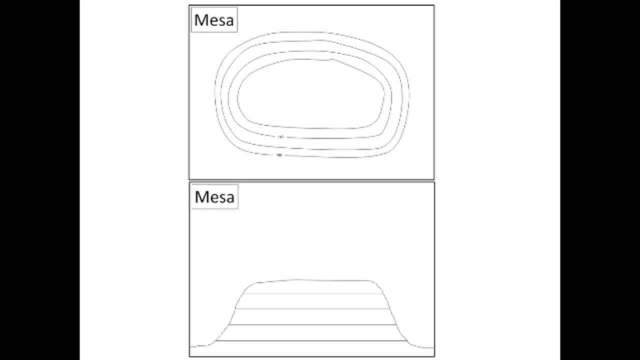 lower than 180. now, a physical feature that I nearly forgot to include in this video is called a plateau. now, what is a plateau? firstly, I'm gonna use this picture of the Mesa to explain it, but you must think large-scale. a plateau is a vast area, it's. it's very, very big. we're. 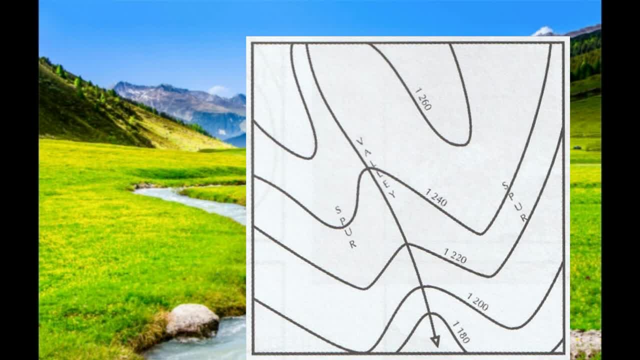 It's not the valley in the picture. It's just a very similar valley in the sense that the slope is very gentle and the contour and the slope is very gentle and the contour and the slope is very gentle and the contour and the slope. 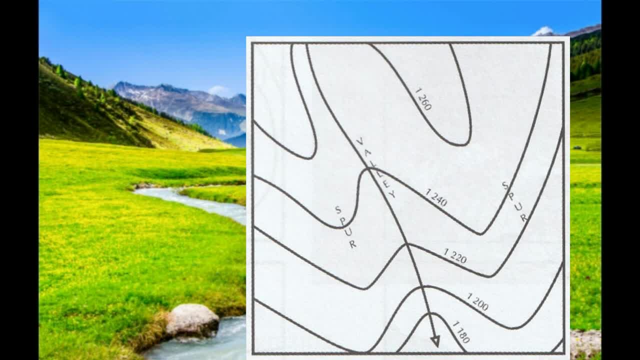 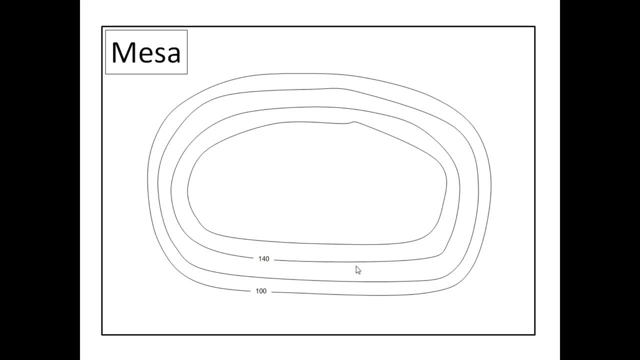 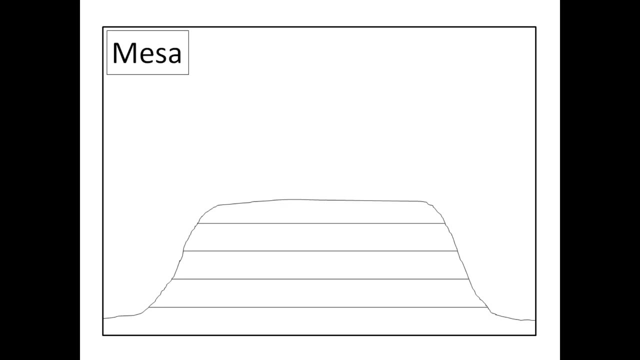 and the contour lines are more dispersed, So it might be slightly more challenging to identify a valley where the lines are so dispersed. Next we have a mesa. Now, a mesa is almost like a hill, but the top is flat, And there we see what the mesa looks like from the side. 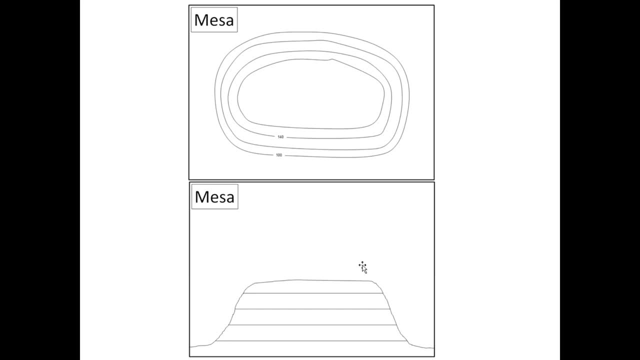 The cross-section perspective looks like this, And there you can see the top is quite flat. Here we see a slope so that the top is smooth, and then on the top there's an angle to the left And there we just have a slope level and an angle to the right. 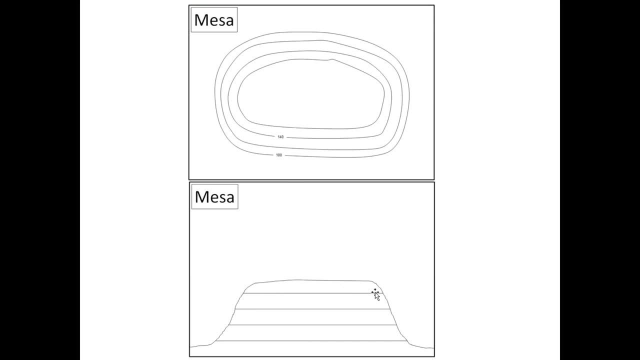 So if this line here were to be sort of above the top, it would be about 160 meters above sea level. But what you should remember- something I haven't mentioned yet- is that if this is there, we see it 140, so this is 160. 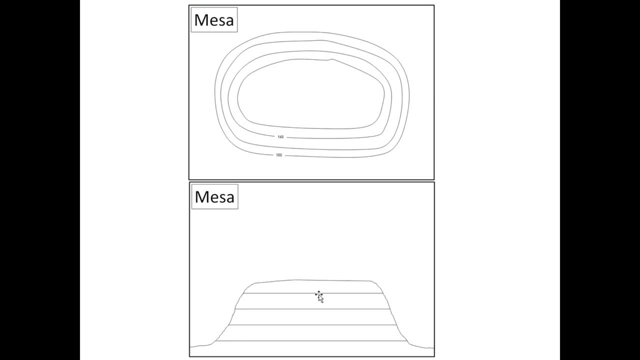 So if this line is 160 meters above sea level, then everything above this is below 180.. And how do we know that? We know it because the contour interval is 20 meters, but we don't have another contour line above this one. So if this line is 160,, 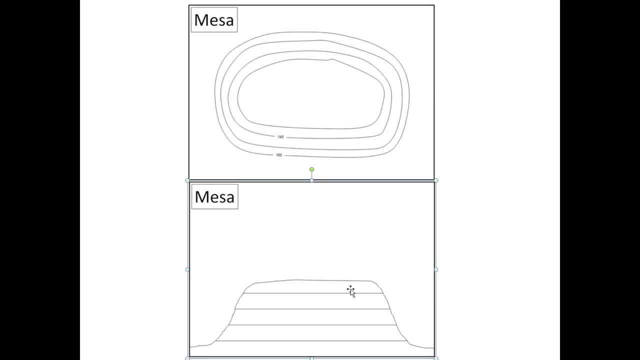 then everything above this is higher than 160, but it's lower than 180.. Now, a physical feature that I nearly forgot to include in this video is called a plateau. Now, what is a plateau? Firstly, I'm going to use this picture of the mesa to explain it, but you must think large scale A. 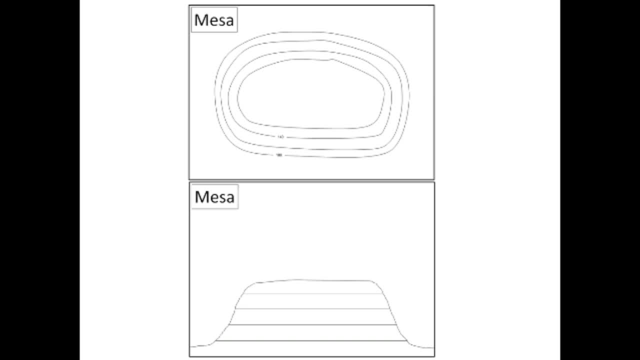 plateau is a vast area. It's very, very big. We're talking hundreds and even thousands of kilometers. So the plateau is that top section that you see, and then what we have is the escarpment. It's where the land rises. So the escarpment is the place that separates high-lying 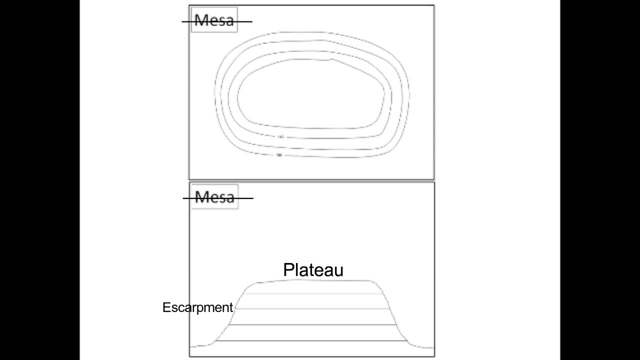 areas and low-lying areas, and how it works is at the bottom section is normally where we have a plateau, and then at the bottom section is where the land rises. So the escarpment is where we have coastal areas, but then from there, as we move inland, what we typically see 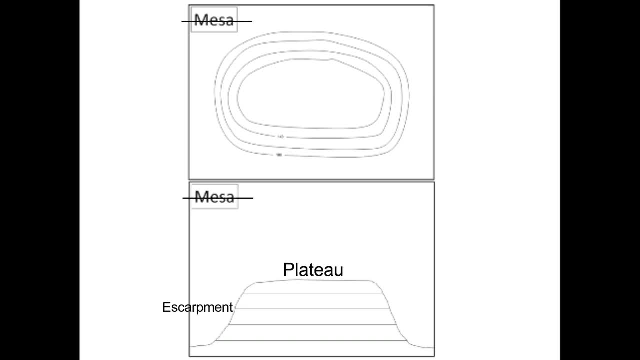 talking hundreds and even thousands of kilometers. so the plateau is that top section that you see, and then what we have is the escarpment. it's where the land rises. so the escarpment is the place that separates high lying areas and low lying areas, and how it works is at the 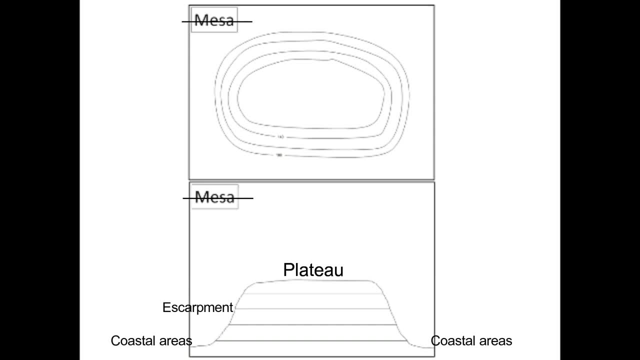 bottom section is normally where we have coastal areas, but then from there, as we move inland, what we typically see is that the land rises and then the interior, the, the central parts of the land away from the. the ocean is where the land is much higher. now we have a volcano. 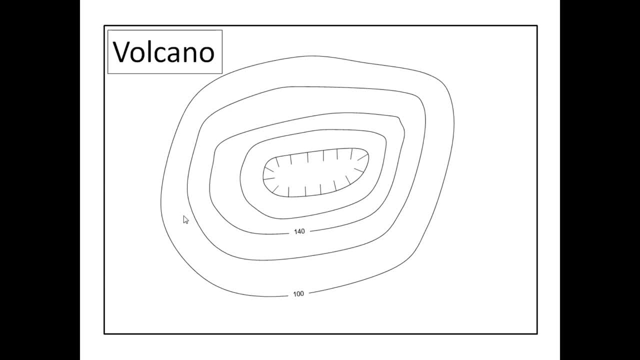 and, as we all know, a volcano is like a hill with a hole at the top, and you'll know when you see a volcano on a map when you see these hatch marks- these are what we call hatch marks- and how it works is as follows: we have a hundred. 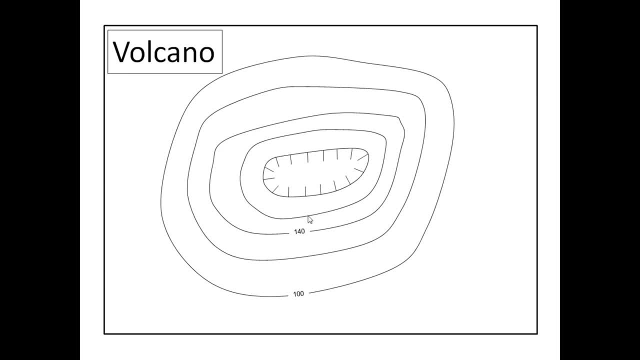 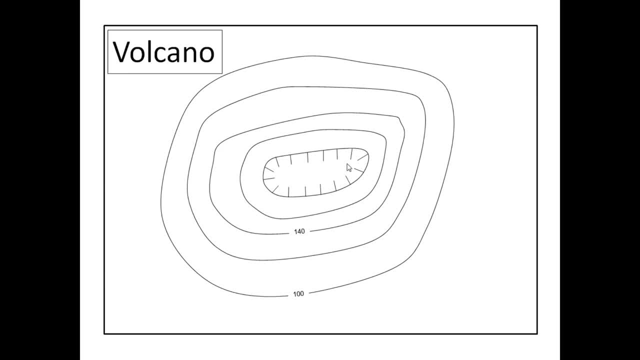 hundred and sixty again. now it is possible to have another circular line in there with hatch marks, and then that would be 140, because now we are going down into the ground. so this is how a volcano is indicated, and the next physical feature is a bit more complicated. what we have here are: 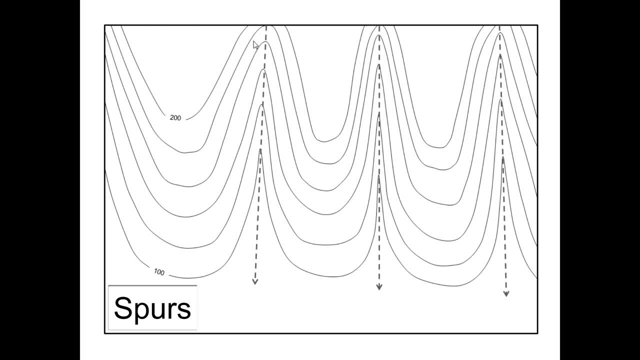 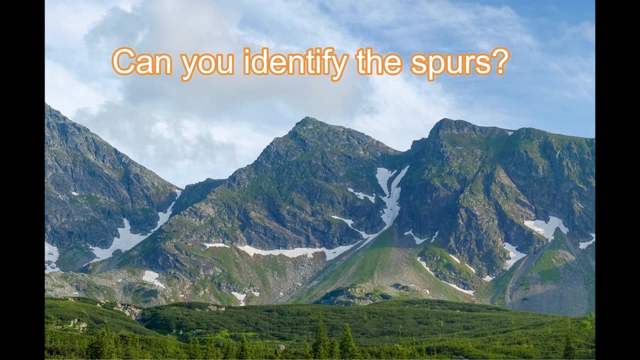 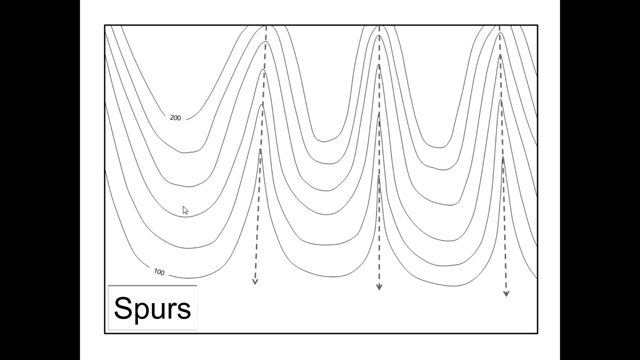 spurs. so this is what we call a spur: this area, as well as this area over here and this one there. so we have three spurs, and how I'm going to explain this to you is that at the bottom or at the foot of a mountain, you will see these. 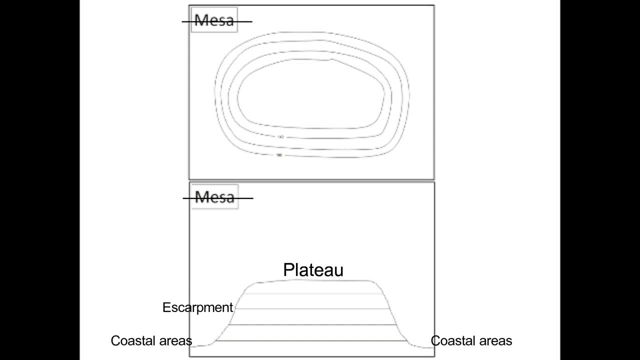 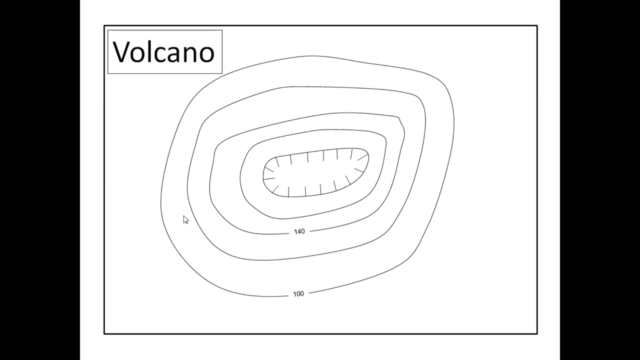 is that the land rises, and then the interior, the central parts of the land away from the ocean, is where the land is much higher. Now we have a volcano and, as we all know, a volcano is like a hill with a hole at the top, and you will know when you see a volcano. 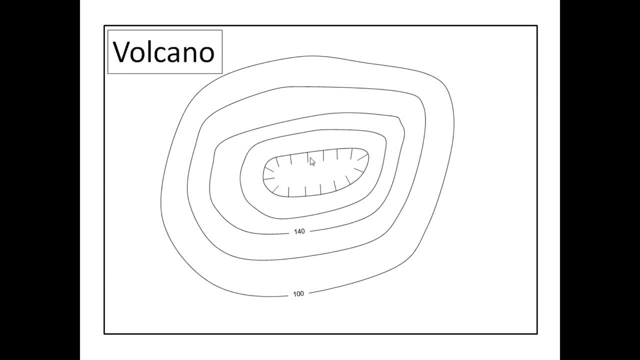 on a map when you see these hatch marks. These are what we call hatch marks, and how it works is as follows. We have a hundred there: 120, 140, 160.. How do we know the height of this line with the hatch marks indicated? It's quite simple. If this is 140, the contour interval is 20, so this: 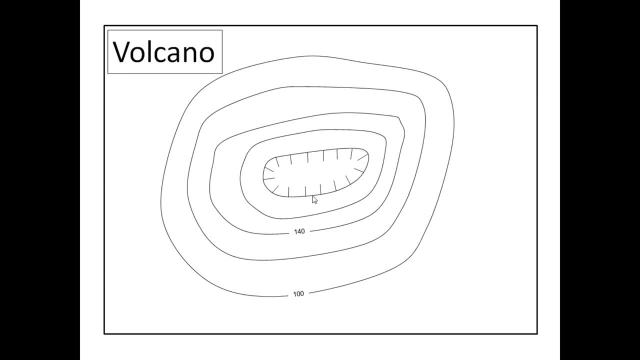 is 160. Then this line is 160 again. Now it is possible to have another circular line in there with hatch marks, and then that would be 140, because now we are going down into the ground. So this is how a volcano is indicated, And the next physical feature is a bit more. 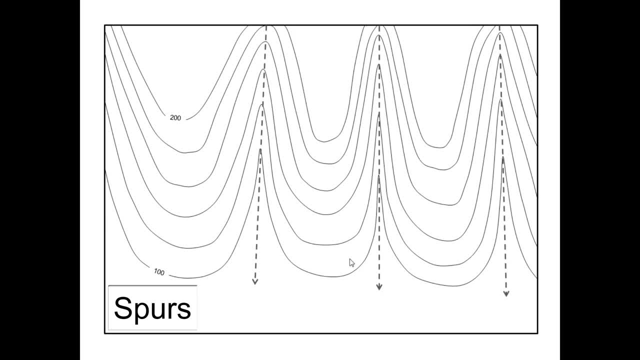 complicated. What we have here are spurs, So this is what we call a spur, This area as well as this area over here and this one there. So we have three spurs, And how I'm going to explain this to you is that at the bottom or at the foot of a. 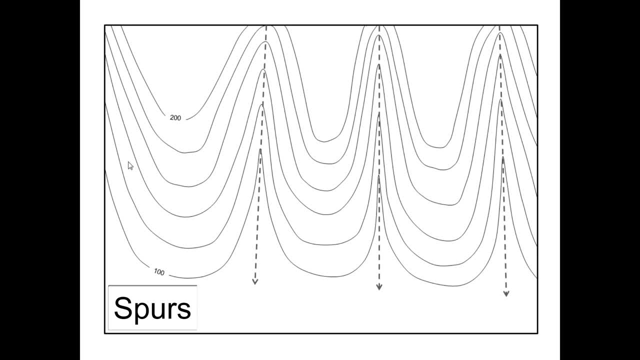 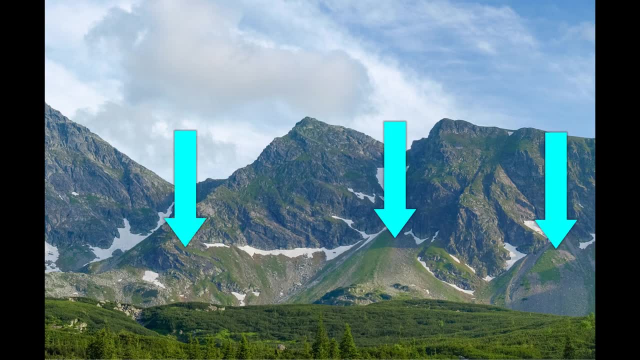 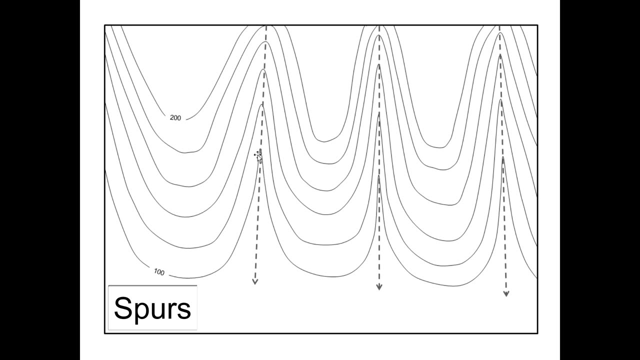 mountain, you will see these toe-like formations. I think you can all remember one of the previous slides. when we have these lines making a V shape, then it points to the source of the river. So once again, there might be a river, might not always be. 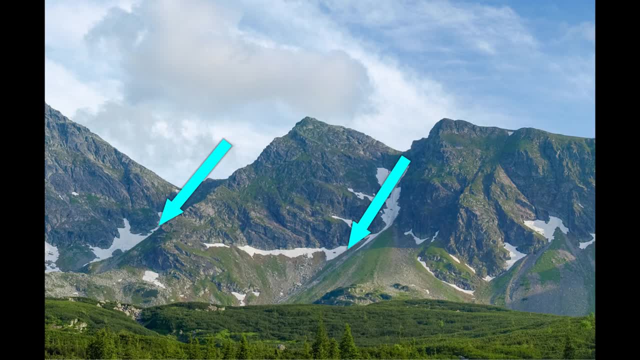 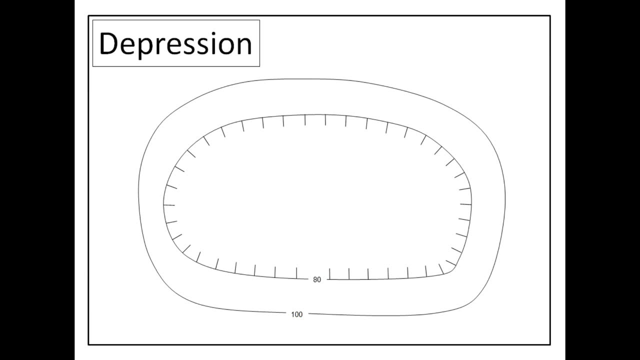 there, but after a good shower of rain, you'll see a river flowing down right there. Okay, so our next physical feature is what we call a depression, and it's basically a hole in the ground Similar to the volcano. you'll see these hatch marks and once again, we are going down instead. 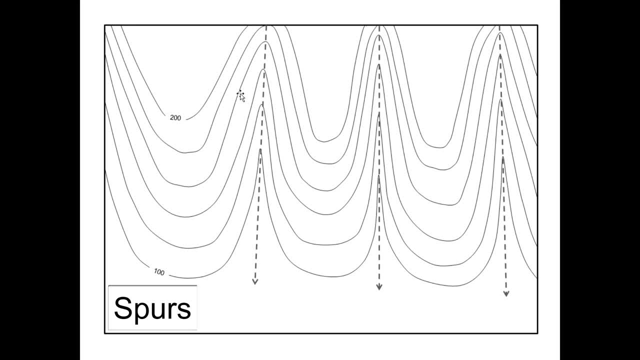 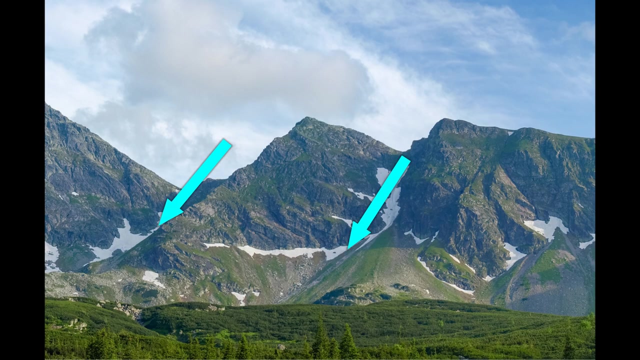 toe like formations. I think you can all remember one of the previous slides. when we have these lines making a V shape, then it points to the source of the river. so once again, there you might be a river. it might not always be there, but after a good shower of rain. 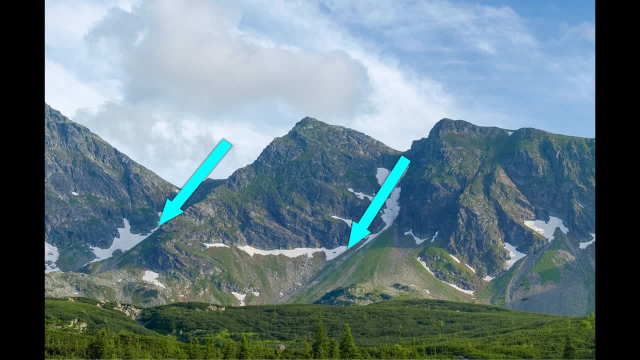 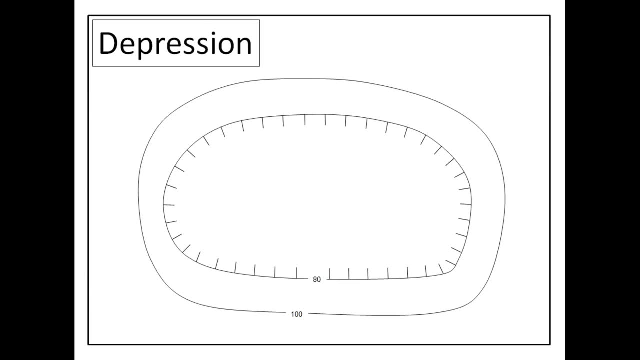 you'll see a river flowing down right there. okay, so our next physical feature is what we call a depression, and it's basically a hole in the ground, so similar to the volcano. you'll see these hatch marks and once again, we are going down instead of up. it could be an excavation site of 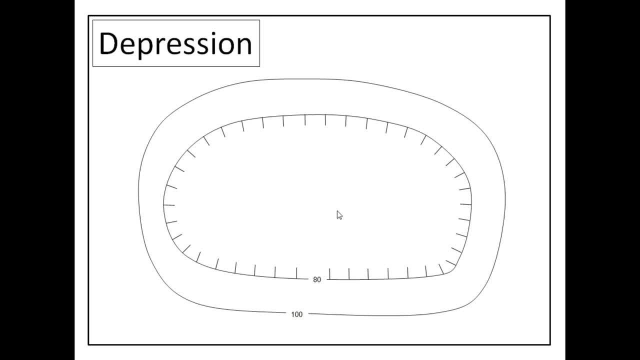 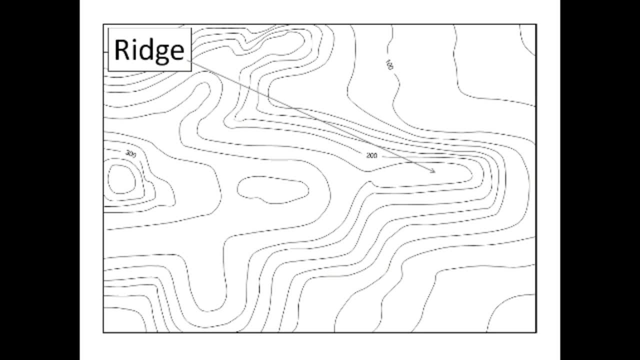 some sort, but it's quite simple. it's basically a hole in the ground. next we have a ridge, and a ridge is similar to a spur in a certain way, but there are a few differences. the first difference I notice is that a ridge is thinner. it's 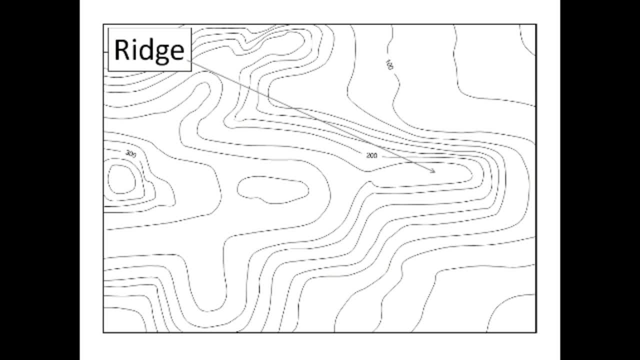 also like a toe, like formation, but it's more like a finger pointing in a certain direction. so it's thinner, the slopes are a lot steeper and here you can see the contour lines quite densely packed. that's where the the slopes are quite steep. but I'm going to show you a picture quickly and please take note. 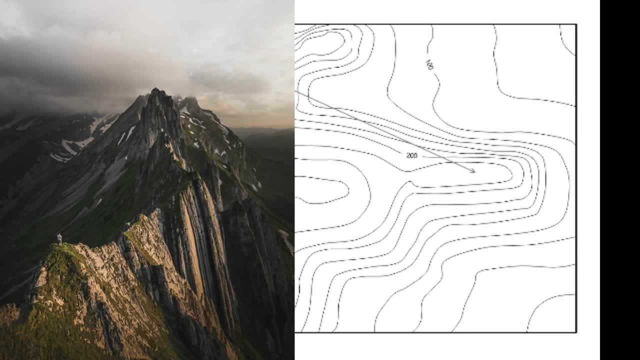 that this is not a physical photo of the contour map. it's just to give you an idea what these things look like. and there you can see the very, very steep slopes. it's very thin along the top of the ridge, but still it gives you a good. 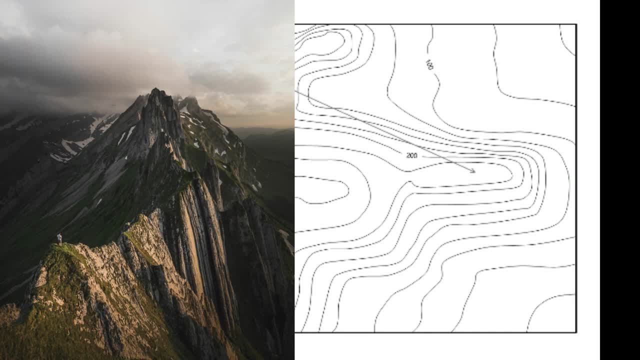 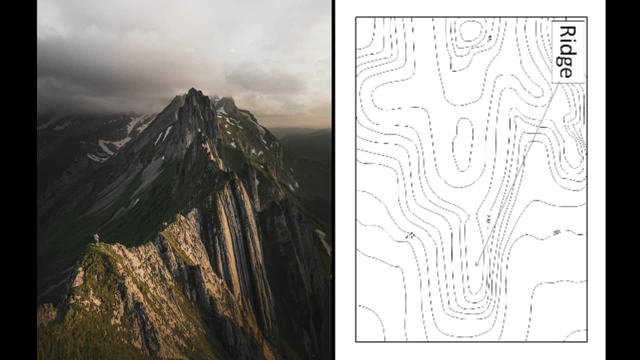 idea of what it looks like. now, just to make it practical, I'm going to flip the contour map vertically just to show you how it looks like, and then I'm going to show you a few similarities, and there we can see how it's pointed it's. 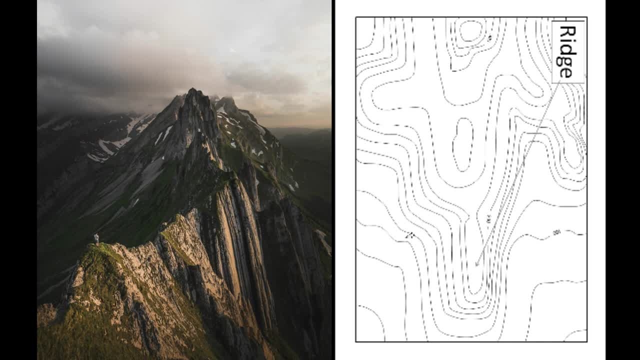 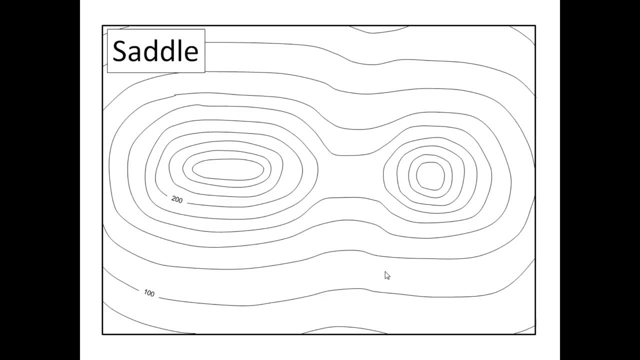 pointing down, in the same way that the ridge in the photo points down, and so this is basically what a ridge is. but let's move on. the next physical feature is a saddle. firstly, we know that these are the lower lying areas, so we're going to go up from a hundred, there's 200, we're going even higher, and then this is: 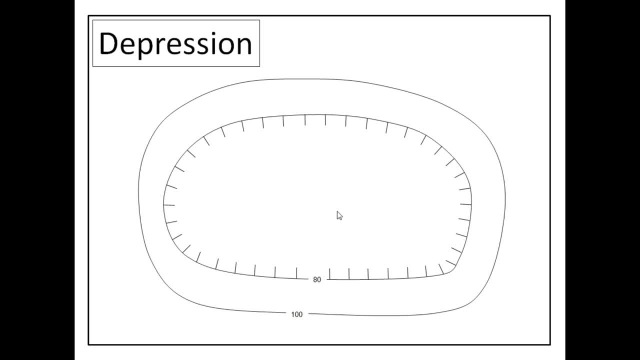 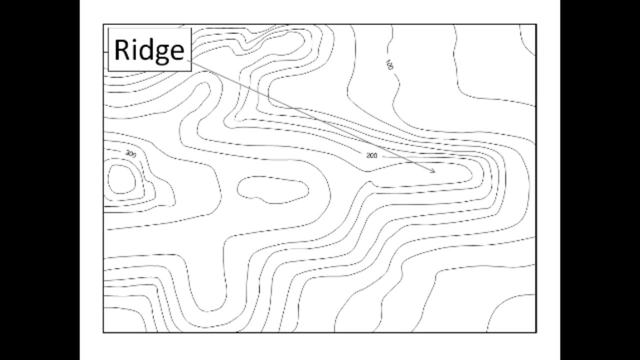 of up. it could be an excavation site of some sort, but it's quite simple, it's basically a hole in the ground. next we have a ridge, and a ridge is similar to a spur in a certain way. but there are a few differences. the first difference, I 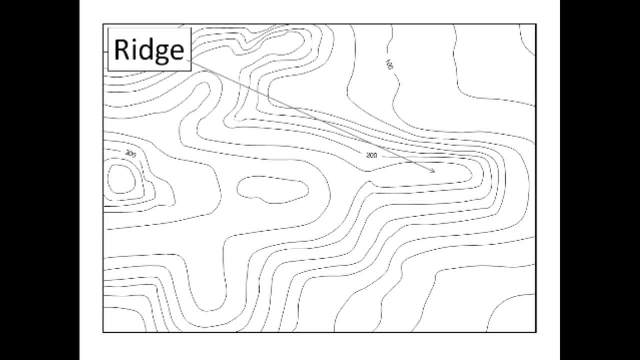 notice is that a ridge is thinner. it's also like a toe, like formation, but it's more like a finger pointing in a certain direction. so it's thinner. the slopes are a lot steeper, and here you can see the contour lines quite densely packed. that's where the slopes are quite steep. but I'm going to show you a picture. 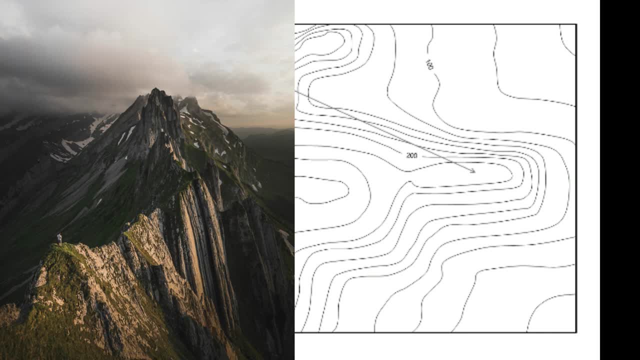 quickly and please take note that this is not physical photo of the contour map. it's just to give you an idea what these things look like. and there you can see the very, very steep slopes. it's very thin along the top of the ridge, but still it gives you a. 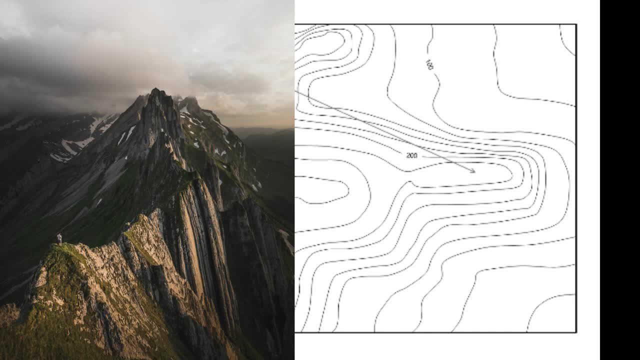 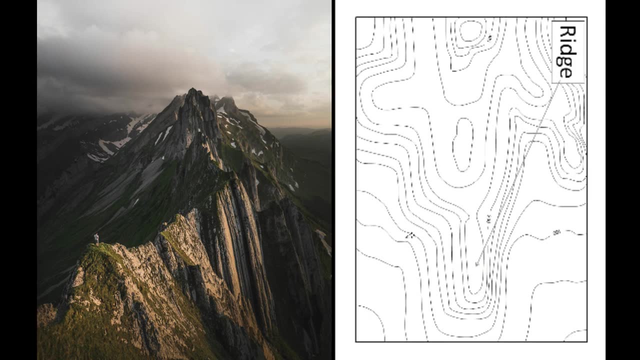 good idea of what it looks like. now, just to make it practical, i'm going to flip the contour map vertically just to show you a few similarities, and there we can see how it's pointed. it's pointing down in the same way that the ridge in the photo points down, and so this is basically what a ridge. 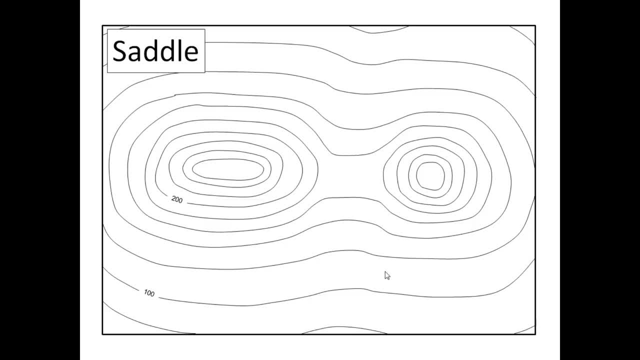 is, but let's move on. the next physical feature is a saddle. firstly, we know that these are the lower lying areas. so we're going to go up from 100, there's 200, we're going even higher and then this is like a hill right. but there we go down again and then we go up again. we will see what. 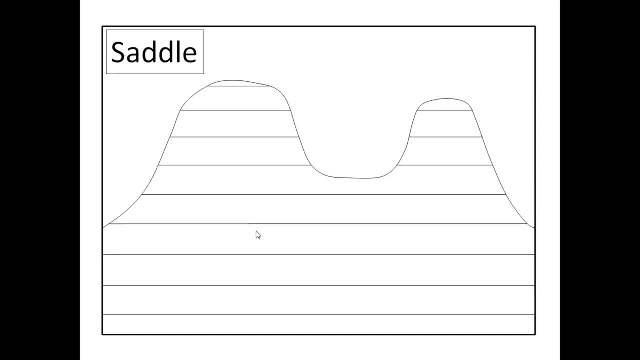 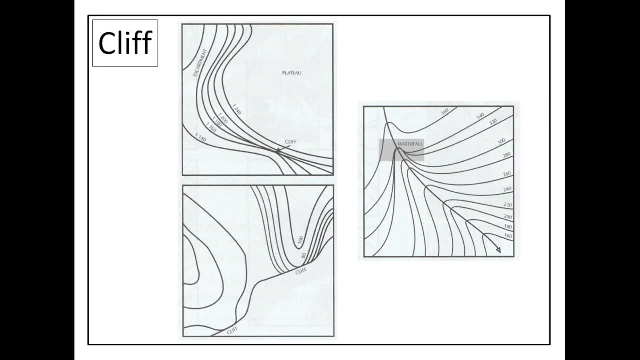 looks like from the side, so please note that the saddle is that dip in the middle. our last physical feature for today's video is a cliff. now, what is a cliff? a cliff is a vertical drop, so it's where the contour lines touch. if we look at the first example, you'll see.